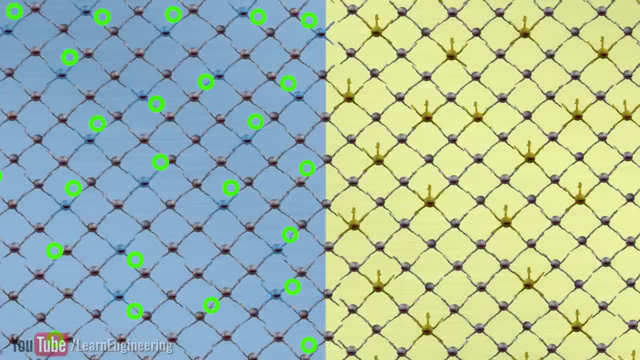 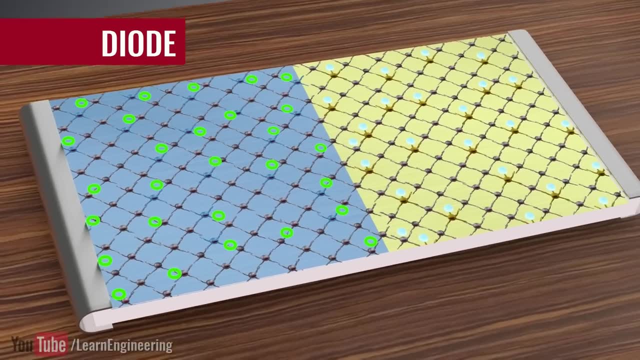 A diode is formed when you dope one electron- One part of silicon as a p-type and the other part as an n-type. Something very interesting happens at the boundary of the n and p-joint. The abundant electrons on the n-side will have a natural tendency to migrate to the holes that are available on the p-side. 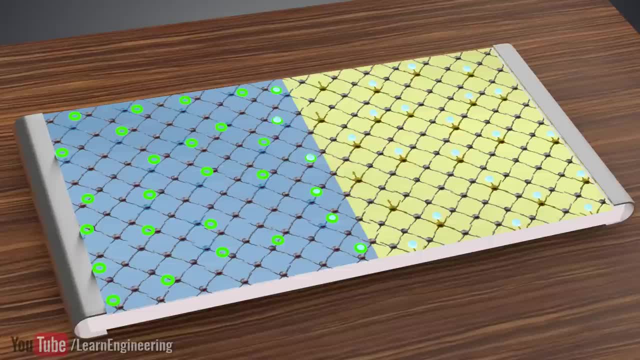 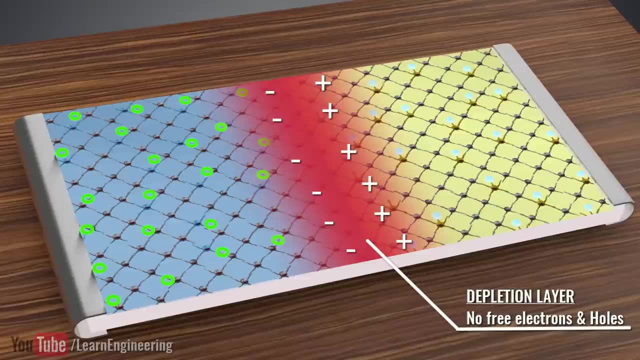 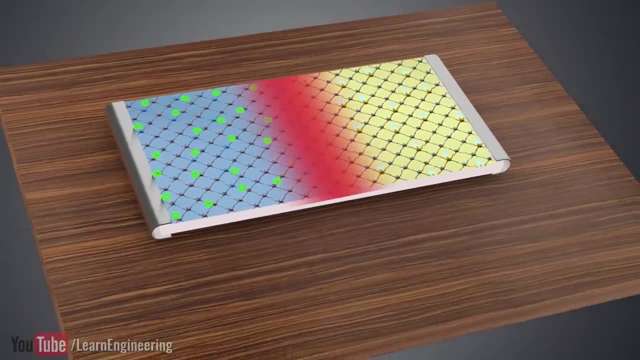 This will make the p-side boundary slightly negatively charged and the n-side slightly positively charged. The resulting electric field will oppose any further natural migration of the electrons. If you apply an external power source across the diode as shown, the power source will attract the electrons and holes. 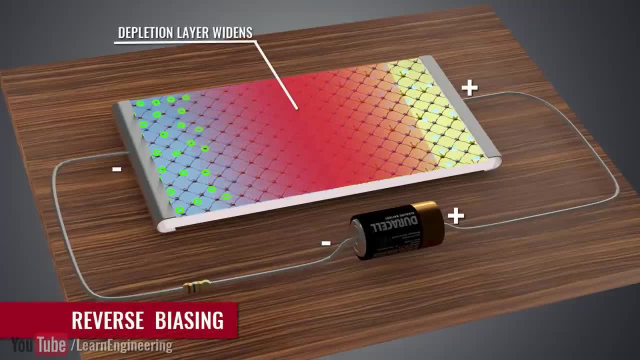 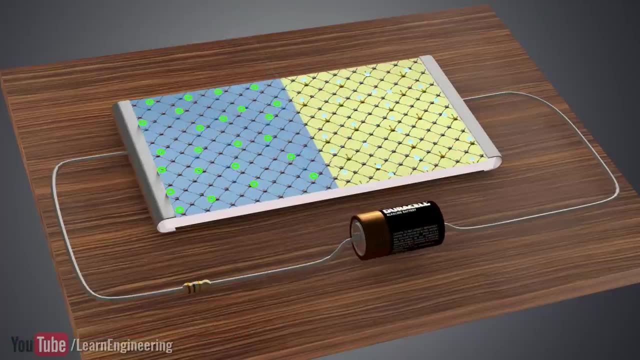 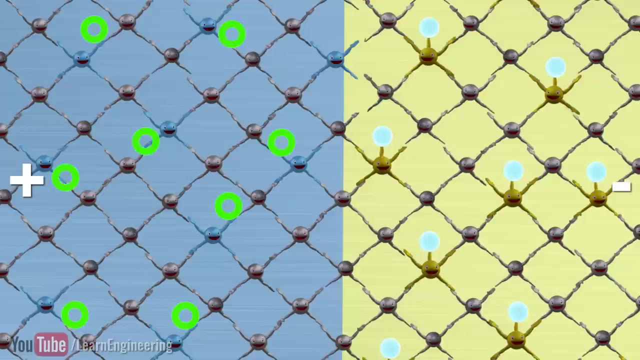 Electricity flow is impossible in this case. However, if you reverse the power connection, the situation is quite different. Assume that the power source has enough voltage to overcome the potential barrier. You can immediately see that the electrons will be pushed away by the negative terminal. 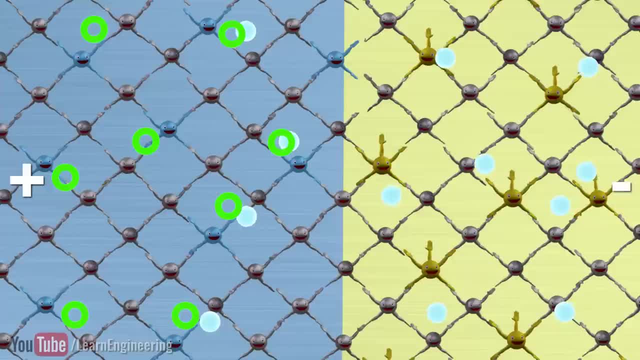 When the electrons cross the potential barrier, they will be drained of energy and will easily occupy the holes in the p-region. But due to the attraction of the positive terminal, these electrons can now jump to the holes nearby in the p-region and flow through the external circuit. 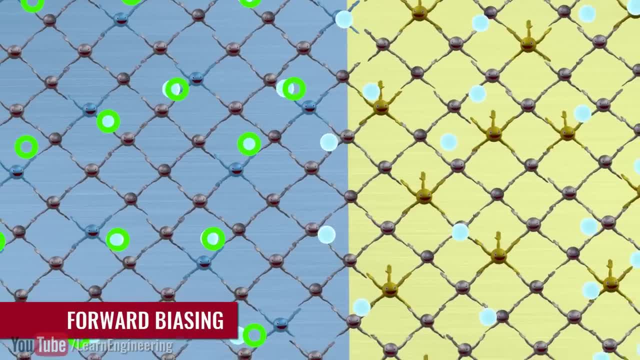 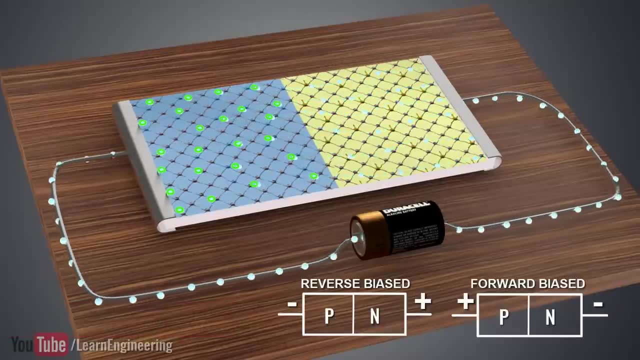 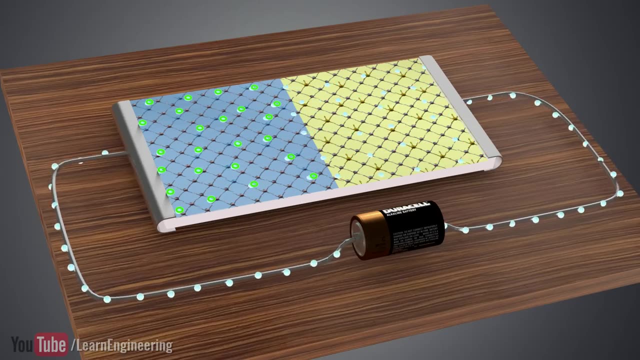 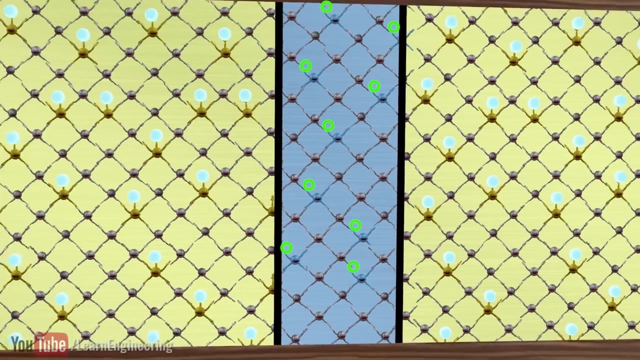 This is known as the forward biasing of a diode. Just keep this simple principle of a diode in mind. You will understand the operation of a transistor very easily. Now back to the transistor. Note that the p-layer is really thin and lightly doped. 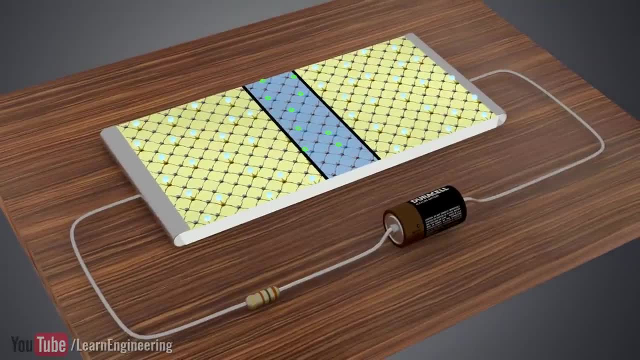 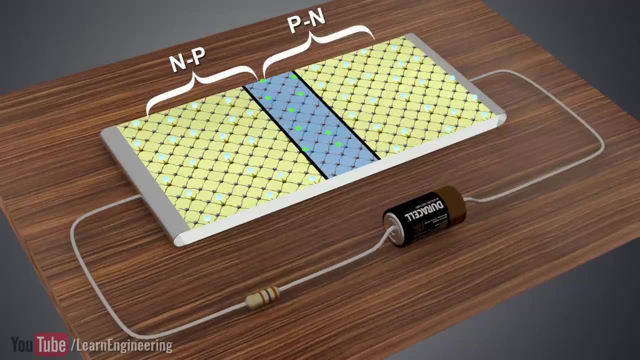 You can easily see that the transistor is essentially two diodes sandwiched back to back. So whichever way you connect the power source, one diode will always be reverse, biased and block the electricity flow. This means the transistor is in the off state. 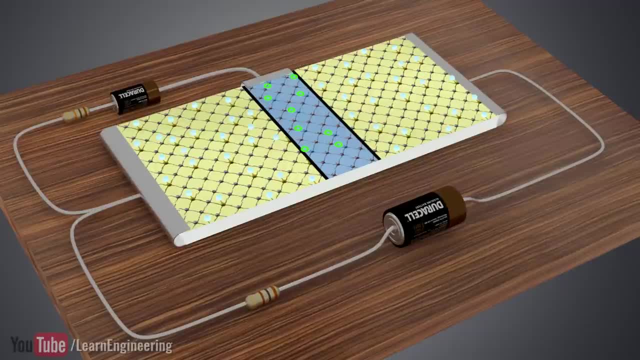 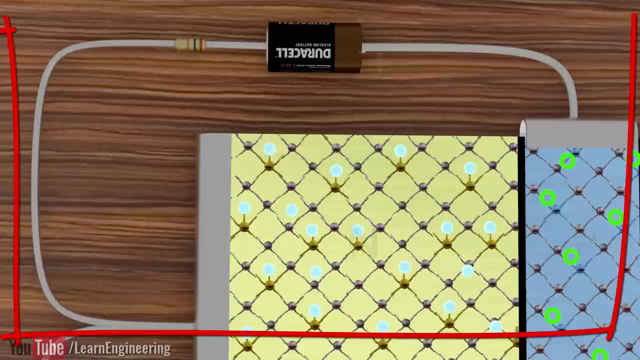 Now let's connect a second power supply as shown, The power supply should have enough voltage to overcome the potential barrier. So this is just a forward biased diode. Thus, a high number of electrons will be emitted from the n-region.